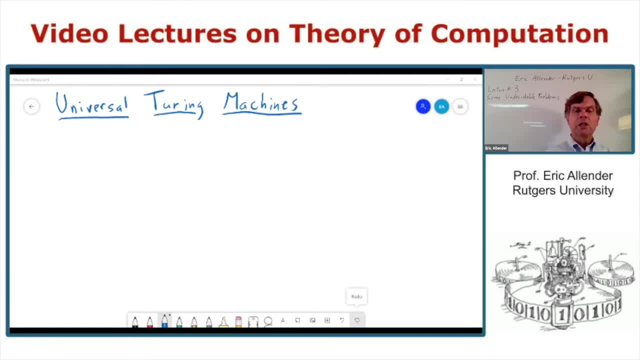 so that shows that the set of valid things is enumerable. What Church and Turing showed was that it is undecidable. So again, we don't know what the answer is. Let's give some other examples of undecidable problems And 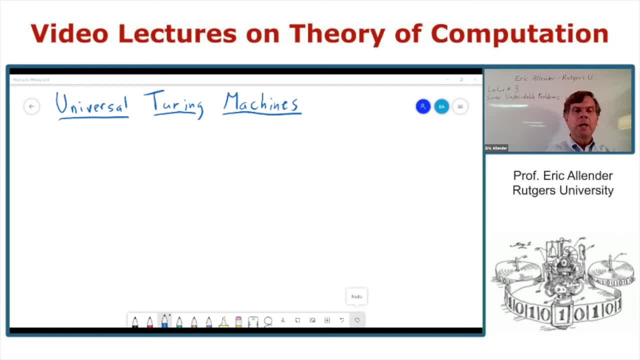 in order to motivate that, the first thing we're going to do is talk about an important notion called the universal Turing machine. So what goes on with the universal Turing machine? what makes it universal? Well, remember, we made the argument that, no matter what, 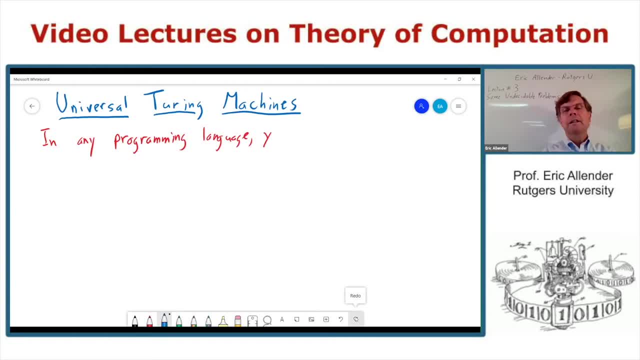 programming language you're working in anything you can do in that programming language. you can also do with a Turing machine, and it's certainly the case that in any programming language you can write a simulator. What is that? It's a program- here I'm calling it SIM- that takes as input the encoding of a program. 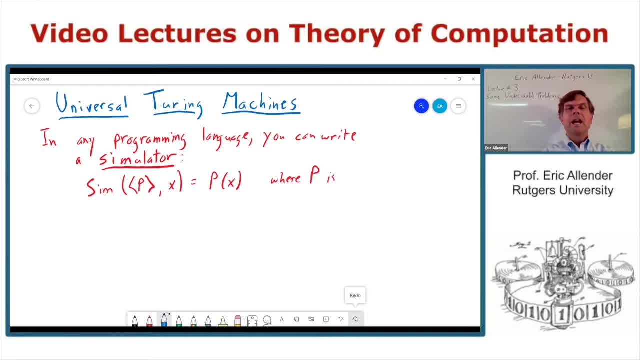 and some string X and you run the program on X. So I'm using these angled brackets, the same way that the textbook does, to indicate that the bit string that represents a program is this P with angled brackets about it, and that differs only in a very slight way from the program itself. 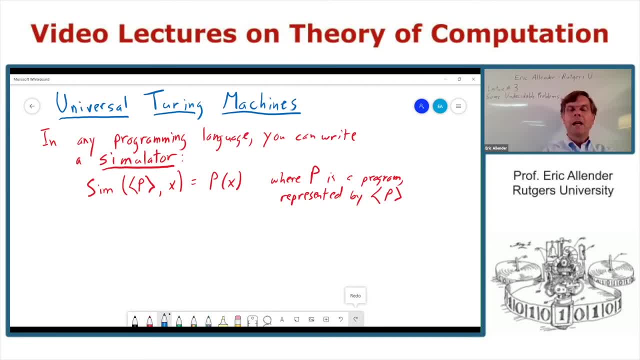 Or the function computed by that program. but it's a just, you know, it's a difference that's being highlighted in the notation that way. So since, if you can do that in your favorite programming language, well then you can also do it with Turing machines, and that machine is called the universal Turing machine. What? 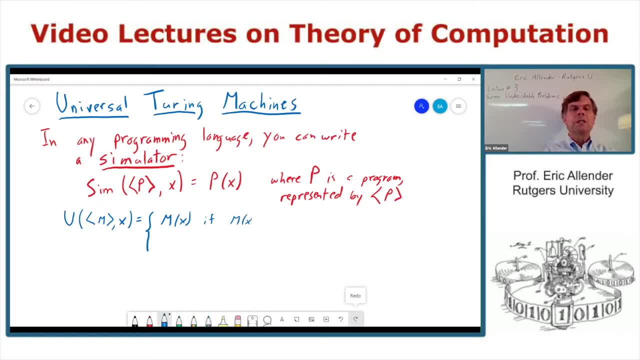 does it do? It takes as input an encoding of a machine M and a string X, and it outputs whatever M outputs on input X. if that computation halts and otherwise we just say it's undefined, which you can think of as meaning the computation doesn't. 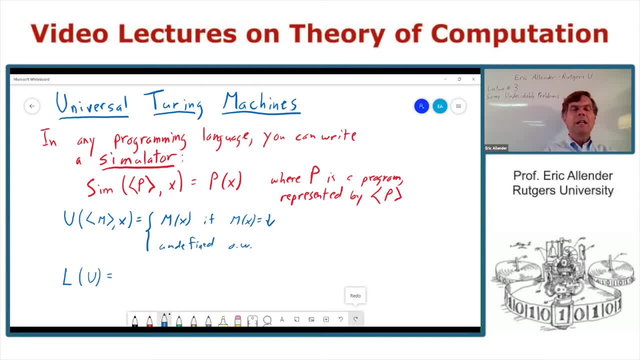 halt Now. this machine, like any other machine, has some language that it accepts and we call that the language of that machine, L, and that has a very special name. we call it A sub T, M, which is those pairs M of X. 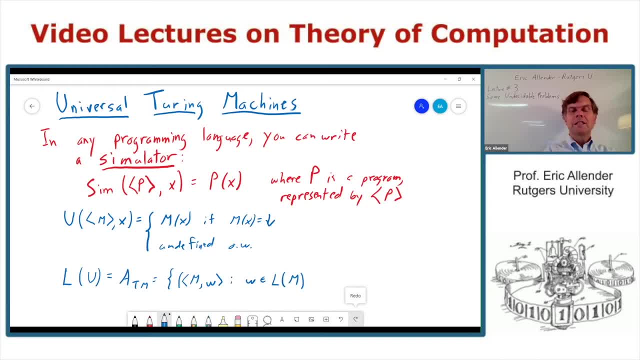 M and X, such that W is accepted by machine M. Okay, so A sub T. M is certainly going to be one of the languages that we'll be working with, and the very fact that there is a simulator is certainly a crucial and important fact about Turing. 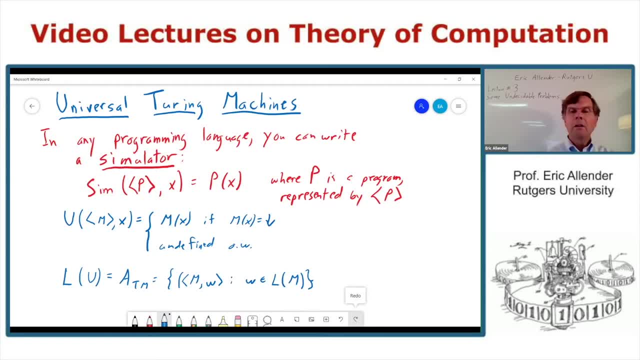 machines. Now let's move on to the question of what are some examples of things that are undecidable. The first thing that we should note before we give any specific examples is that there are only accountably many programs, because what is a 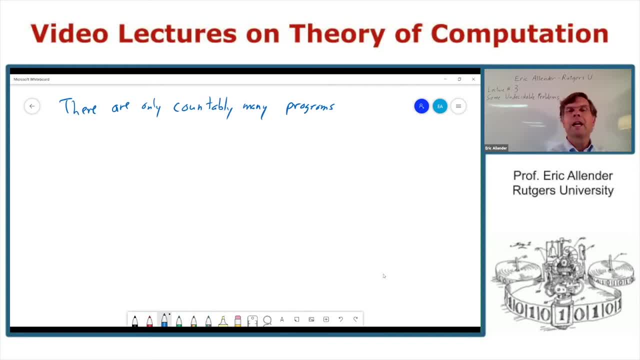 program. a program is just a something you can write down, so it's an element of sigma star, and sigma star is a combo set um, and so this is also certainly true for turing machines. there are only countably many turing machines, uh, but there are uncountably. 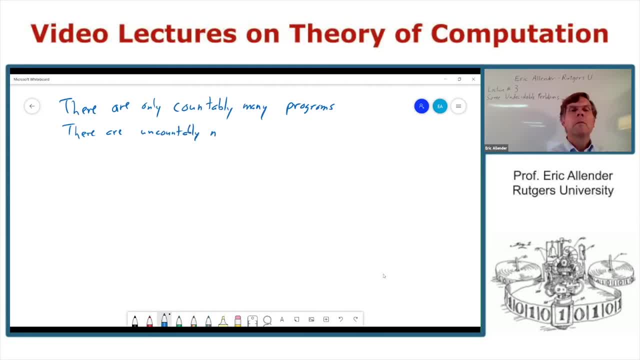 many subsets of the natural numbers, or of zero, one star. in other words, there are uncountably many languages, so in some sense hardly anything is computable. there are just way more languages, way more functions than there are programs, so hardly anything is computable. but that's not. 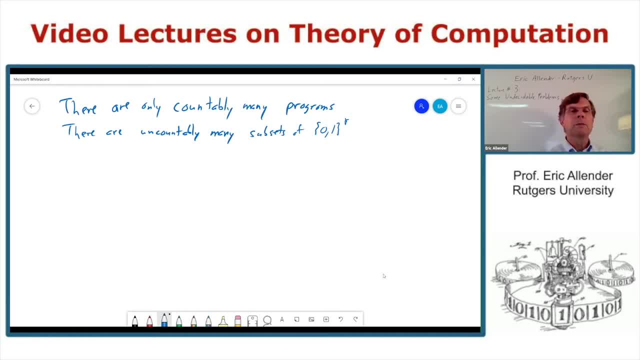 near enough to be true for a turing machine. so there are many subsets of the natural numbers so interesting as to know some specific examples, And one famous example. one important example to know about is the halting problem. There are different versions of the halting problem. We're going to define it as being the set of 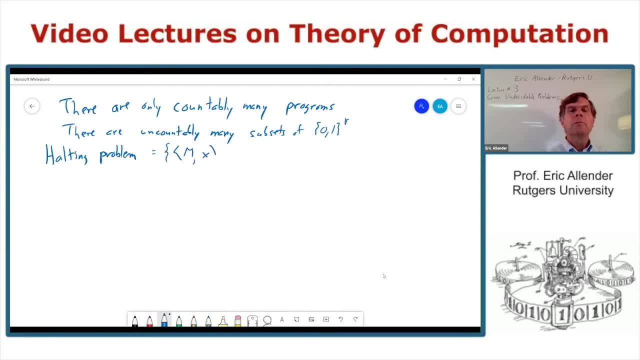 all machines M and inputs X such that M on input X halts. Different texts would define this as being the set of all those machines M that halt on their own input, on their own encoding, And I don't want people to freak out when they 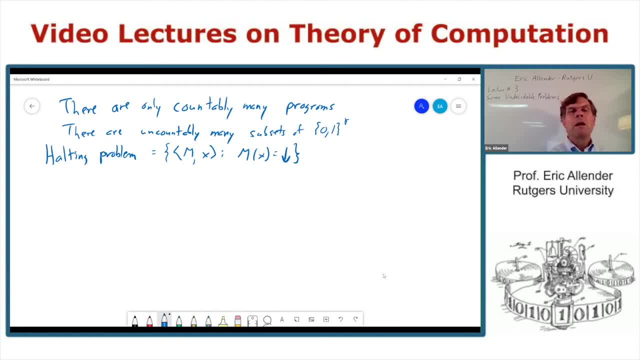 always encounter these examples about programs being run on their own code, because this is a problem, And I don't want people to freak out when they always encounter these examples about programs being run on their own code, because this is something that happens all the time. There are a lot of programs that take 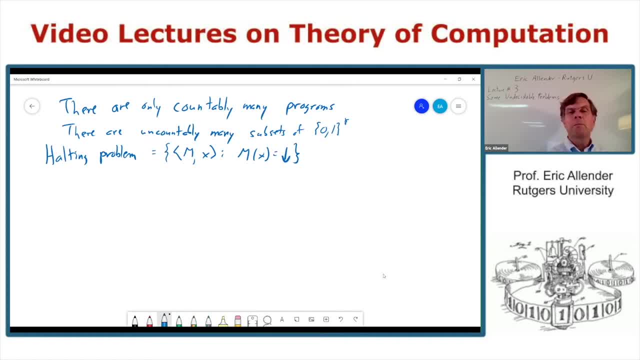 other programs as input. Think about compilers, for example. If you've got a Java compiler, you can write that in Java and you can use that compiler on its own code to compile its code. So there's nothing really weird about having programs run on their own input. It happens all the time And we will. 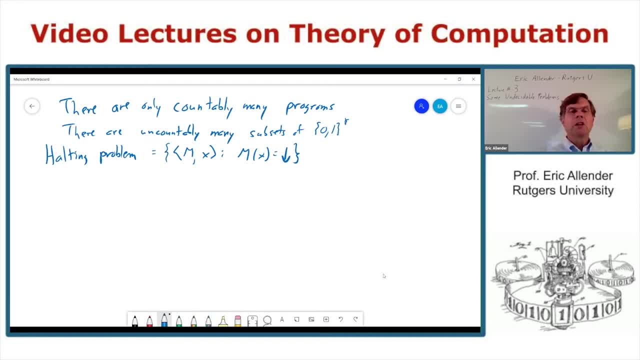 certainly be seeing other examples which maybe do look a little bit weird. So I will claim that the halting problem- let's just call it H- is recursively enumerable. It's Turing acceptable. Why is that? Well, you take as input M and X. 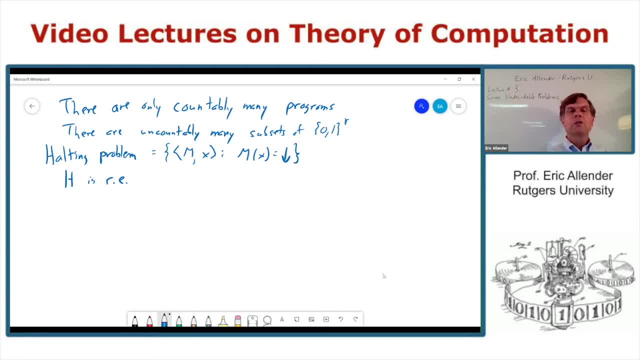 you run using our universal Turing machine. you run M on input X, and if that computation ever halts, then you run M on input X, and if that computation ever halts, then you run M on input X, You go to an accepting state and otherwise, of course, if it doesn't halt. 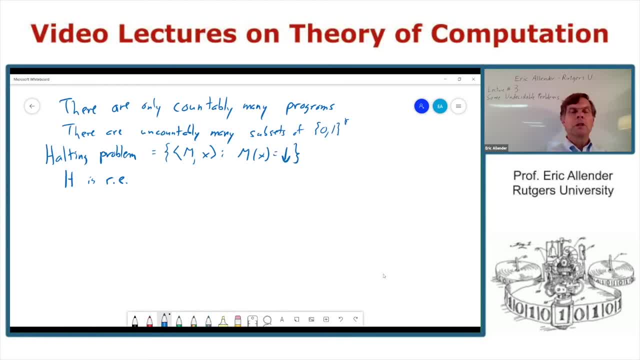 there's nothing to worry about. You will never halt and, in particular, you will never accept. So it's definitely Turing acceptable, but it's and it's not decidable. decidable, which means that H complement is co-RE and not RE. okay, So almost all of the examples that 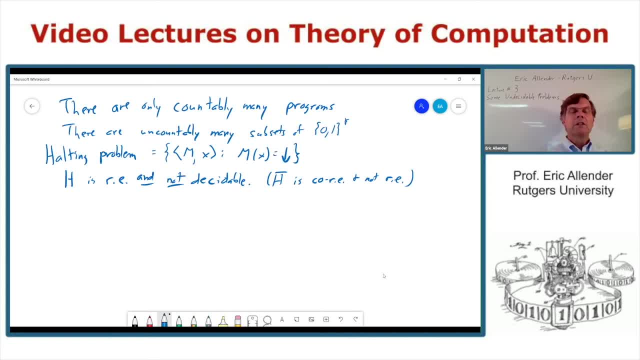 we will be giving. well, in fact, every example that we'll be giving in this lecture is going to be something that is computably enumerable and not decidable. therefore, its complement is co-RE and not not CE. Okay, so how do we prove this? 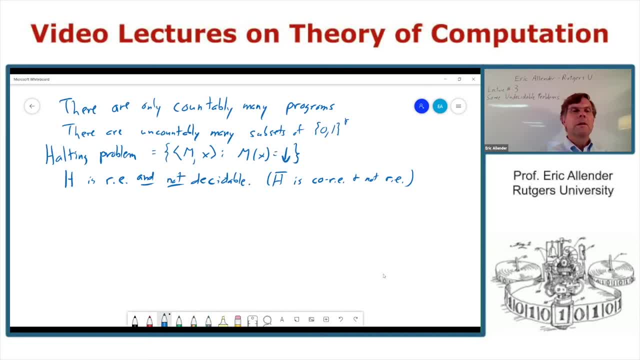 This is a theorem. It'll be a proof by contradiction. Assume otherwise. so, in particular, assume that halt is some subroutine, some program that decides H. Well then, consider the following program, which I'm going to call bad. Bad takes input the encoding of a machine, M, and what does it do? It runs program. 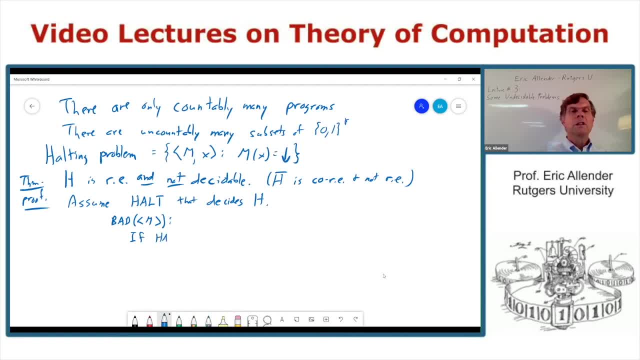 halt. So if halt that subroutine, that magic subroutine on input M, comma M, says yes, then this program will loop forever and otherwise it will halt And let's say halt and accept whatever. Okay. so this is a program and like any program it can be represented by a bit string, and I'm 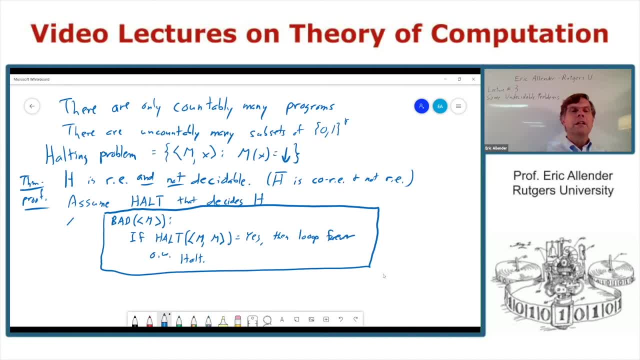 going to call this bit string B, the encoding for that program B. So the question now is: does program B halt when it's given its own code As input? Remember it's a program. you can run it on any kind of input, including. 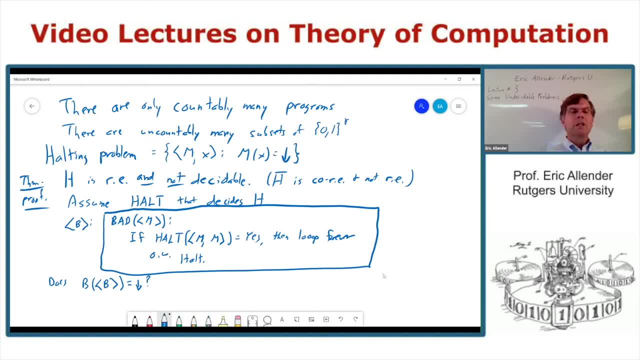 its own program, and I'm using this down arrow to indicate halt. So this is the question, and note that if the answer were yes, well then what's this program do It goes? remember we're running B, which is this program on its own code. 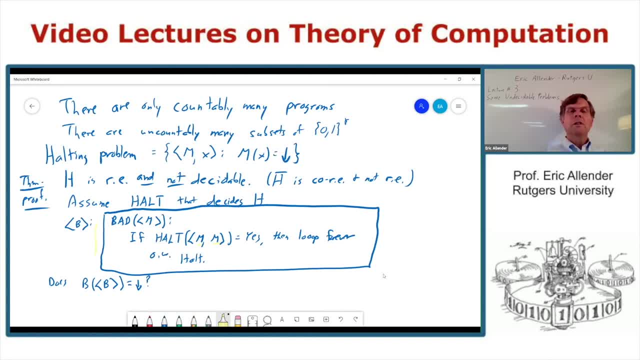 and if it does halt its program, by definition is going to output yes, which means that this program B will loop forever, which means that if the answer is yes, then the answer is no. So that's impossible. So that means that the answer is no, but if the answer is no, you. 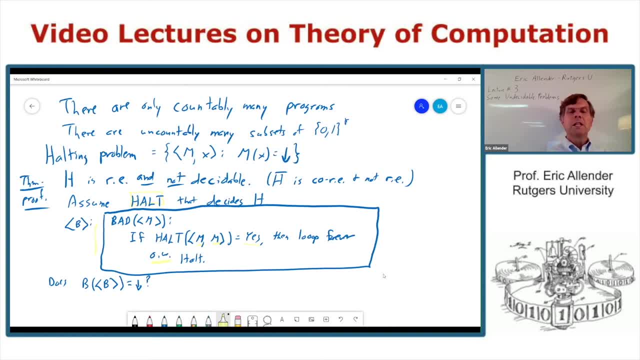 go down to the otherwise or the else part of this statement and you halt. So if the answer is no, then the answer is yes. That's a contradiction. So in other words, this program is nonsense. It can't possibly exist, but it does exist. 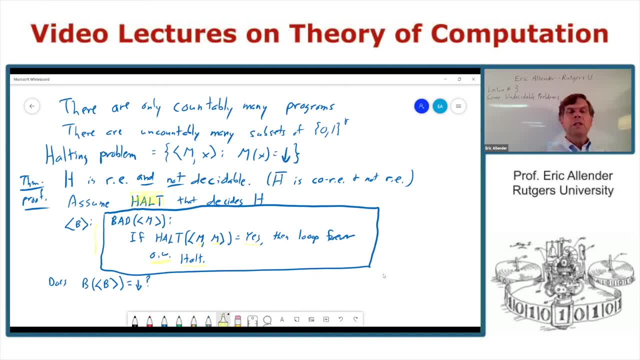 assuming that halt is a routine. In other words, if there's a Turing machine, if there is some decidable algorithm that halts and actually decides the language H, So that means it's not decidable. So good enough. What's something else that we can now? 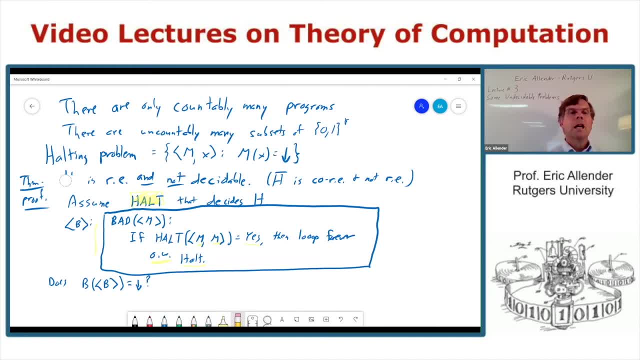 say is not decidable. Let's look at A sub Tm. We're going to claim that this is recursively enumerable, computably enumerable and not decidable, which means that it's complement A sub Tm. Okay, A sub Tm is co-Re and not Re, So we're going to assume that A sub Tm, let's call it, except. 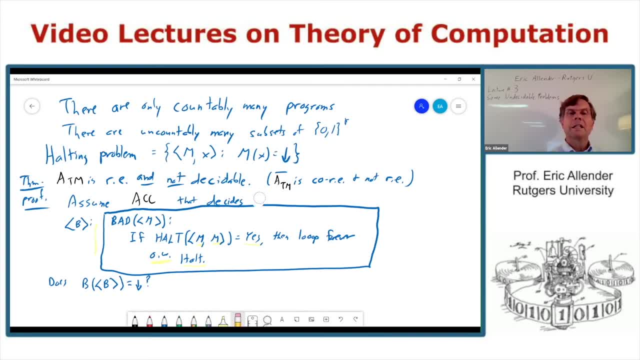 is some subroutine that decides A sub Tm. Now what does that program look like? Again, we're going to call it bad on input M. if Now we're going to call, except on this input M, M is yes And we're going. 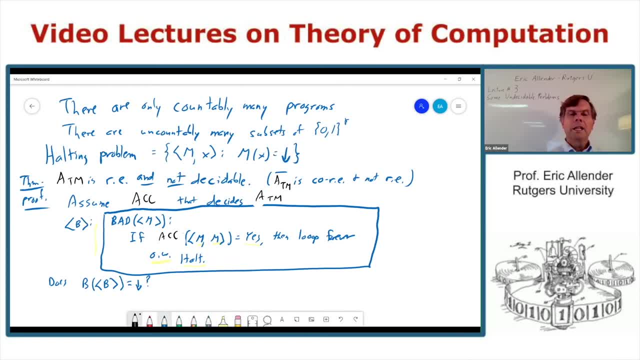 to call it instead. And if so, when we define X equals to X, it means that we label a subroutine that stops and returns yes when different parameters of T are functioned within it. So assign something else when I set it up to sort of myselfки. 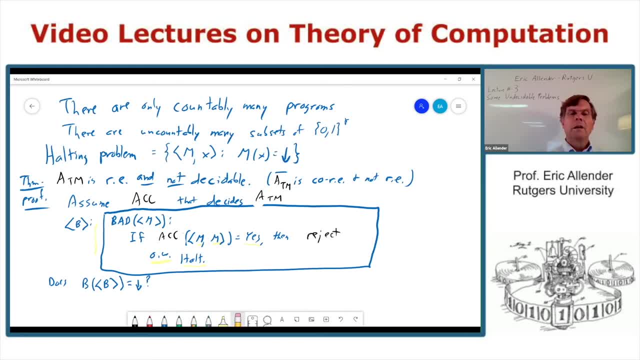 and an external letter. So if I'm gives possibilities and we're Blowback and returns yes or no, Then this routine bad is certainly something that we can write. and now let's call this piece of code b, and the question is now: is the encoding of b in the language accepted? 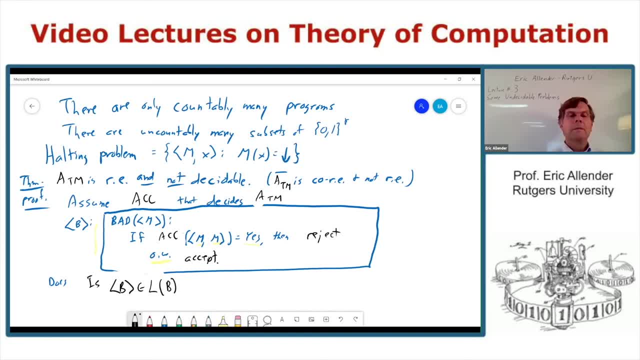 by that machine b. Well, what do you think? If it is, then our subroutine x is going to say: yes, this program that we're looking at b accepts if we run it on input b, and in that case we reject. So if it is accepted, it's rejected. so that can't happen. Therefore. 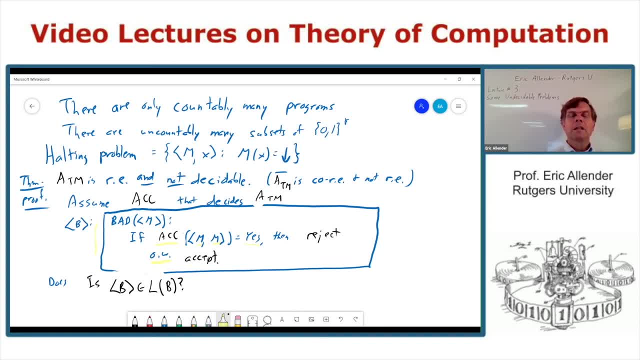 the only possible possibility is that it's not accepted, which means that this is going to return. no, which means we've gone down here to the otherwise and we accept. So if it's not accepted, then it's accepted Again. we get exactly the same contradiction. 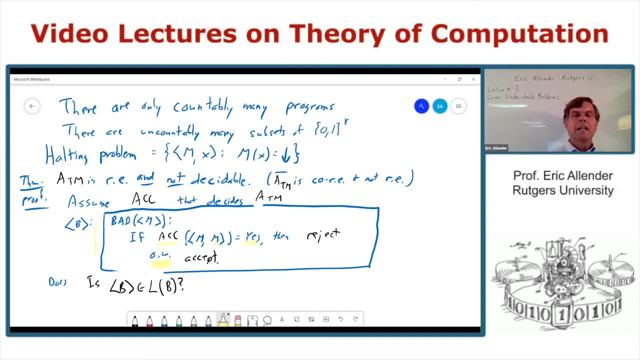 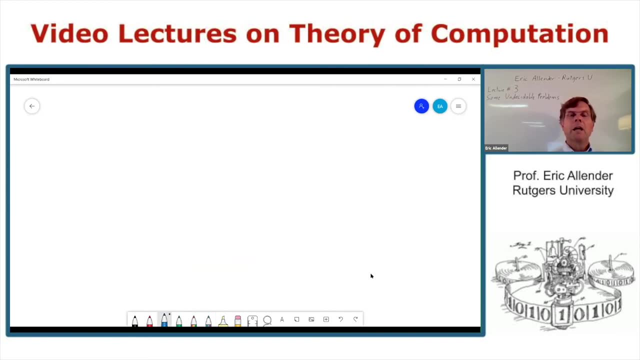 So there you have it: yet another example of something that is Turing acceptable and not decided, Thank you. So remember this handy-dandy diagram where we have the computably enumerable sets and the co-computably enumerable sets. We've shown that the halting problem and a sub t, m and 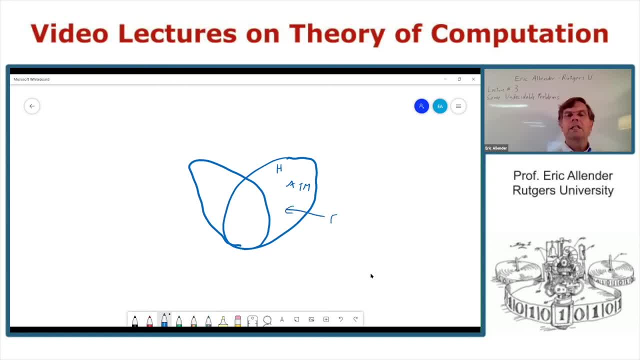 actually also don't have room to write it here, but the enscheidungsproblem, you know. the set of valid formulae: maybe I'll just call that v, The set of first order statements that are valid. those are all here, whereas their complements. 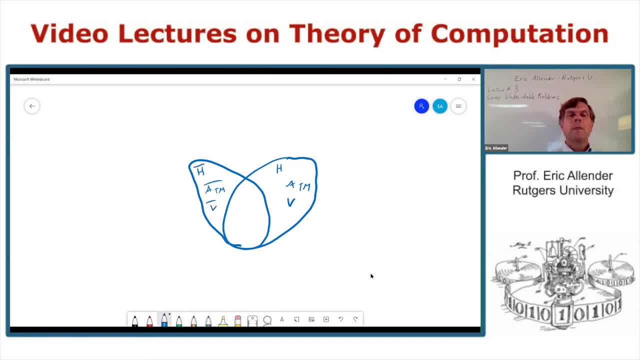 are all over here, And later on in a subsequent lecture, you will learn that in some sense these are actually all the same problem. In other words, given an instance of one, you can transform it into an instance of the other. For instance, if I don't have a set of first order statements, 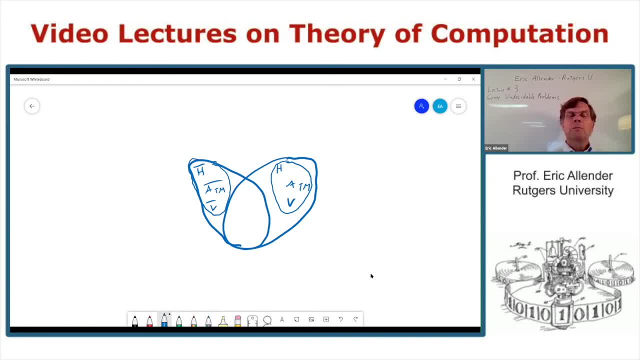 I may not have a set of first order statements that are valid. Those are all here, whereas- and all these problems are what is known as complete. You'll learn an important vocabulary word about completeness, and that will happen in a later lecture, So let's just recap where we have. 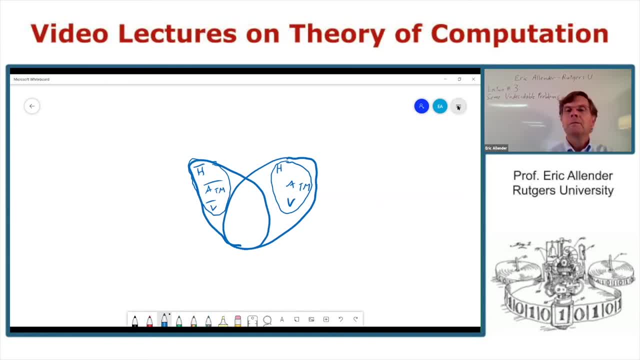 been in the last few lectures. We've started with what you learned about in the previous lecture about Turing machines and note that there is sort of a robustness to the definition of Turing machines. Just about anything that you would like to tweak the Turing machine model to get will give. 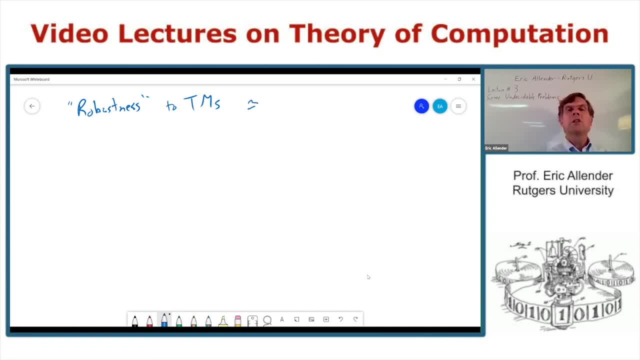 you something that's equivalent to Turing machines and basically it's also going to give you something that's equivalent to programs, And certainly we're familiar with the notion that there are tons of different programs out there- programming languages, and they're all equivalent. Turing machines are really in some sense, just 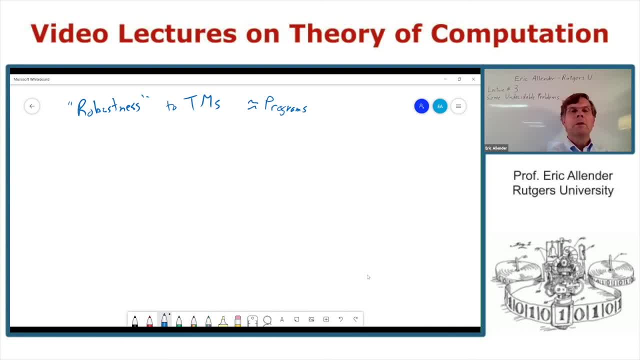 another sort of inconvenient programming language, but they have the advantage that they're very simple to work with. We learned about the church Turing thesis And that the real meat of the church Turing thesis is just this statement that no matter what notion of programs you 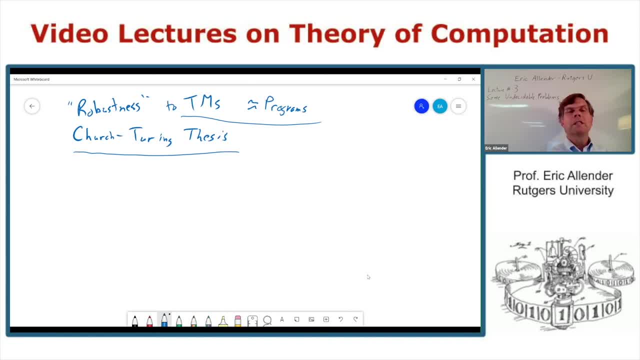 come up with. it's gonna be something you can implement on a Turing machine, And an important corollary then is that if something is not computable by a Turing machine, particularly if it's not decidable or if it's not even Turing acceptable, then constructed incapacitation of programs will be an�p. 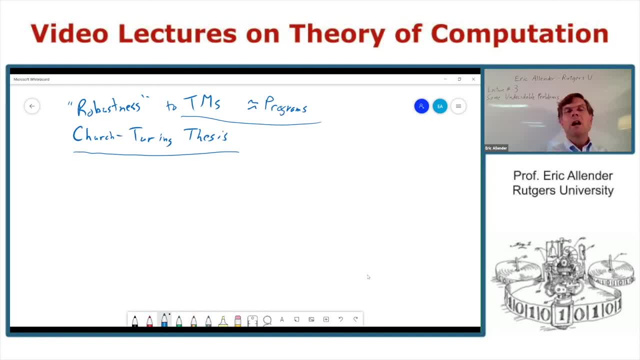 it's not going to be decidable or acceptable. on anything else that you come up with that looks like it ought to be a notion of computation that you can actually implement. This was something that will never be proven, but it's something that is pretty widely accepted in the community.